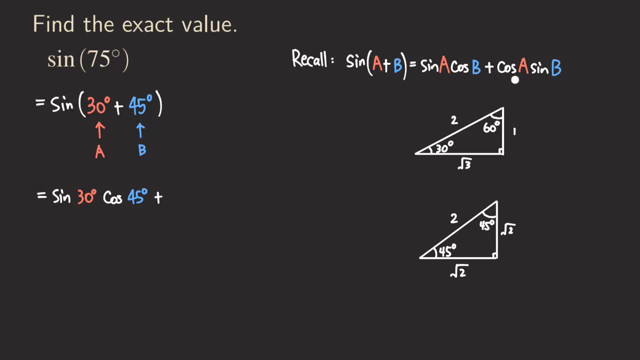 And then plus, and then plus the next one cosine of A right Cosine A, cosine A would be 30. And then the next one would be sine of B. B is 45. So we are going to get 45 over here. So now we actually have applied the sum formula. The next step is to actually find the value of each of those sine 30, cosine 45, cosine 30, and sine 45 degree. How do we find the value of each of those sine 30, cosine 45,, cosine 30, and sine 45 degree? 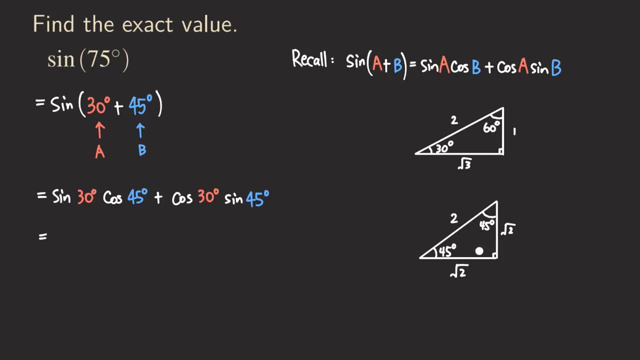 So we find that we can actually just refer to the two special right triangles. And since all those quadrants are in quadrant one, then what we need to do is to just worry about finding the ratio. we don't need to worry about the signs anymore. all those are positive right. So we are going to get sine of 30. So sine of 30 is the looking at this angle. 30 over here. it would be what opposite over the hypotenuse. So it would be one over two. So our first number for 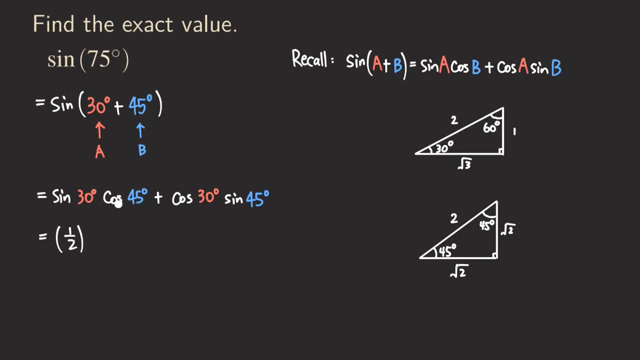 this term. first factor would be one over two. cosine 45 degrees. So if we look at the cosine 45 degree we get it. look at this angle or that one doesn't matter. So for cosine 45, we are going to look at the what, the adjacent over the hypotenuse. so it will be radical two over two. So we have radical two over two, then plus and then now the next one. this is the first factor, the second term. So we are going to get cosine 30. 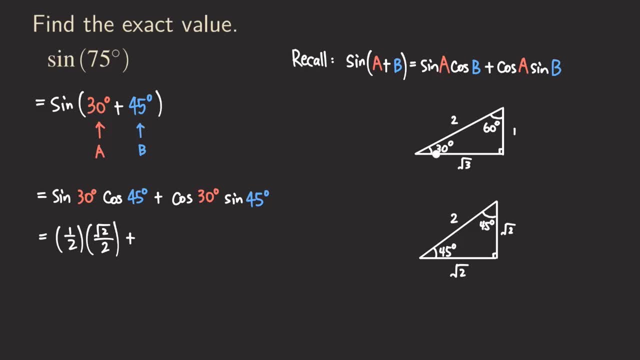 degrees. So we are going to look at this one. So cosine 30 degree, it would be what? adjacent over the hypotenuse? So radical three over two. so we are going to get radical three over two. and then times sine, 45 degrees. So looking at the 45 opposite over the adjacent, so radical two over two, so radical two over two. So now we actually have the value for each of those expressions right here. Now, multiplying those two together, we get radical two over two. plus what about this one? 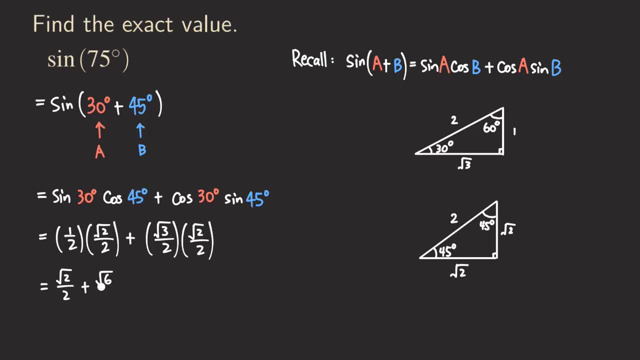 radical six, radical three times radical two is radical six over- well, four. actually I was going too fast, So that would be four and four here. two times two is four, And so now that is the final answer. Or, if you want, you can put it as a single fraction, So it would be radical two plus radical six, and then over four, And so that's that Okay. And then now let's look at the next example. 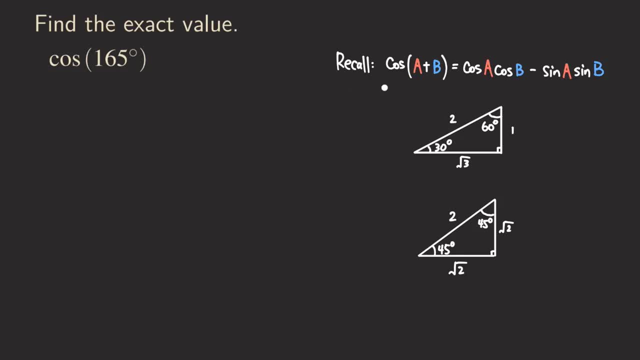 Okay, In the previous example we use the sum formula for the sine. This time we are going to look at the sum formula for the cosine, But we can also use the difference formula for this. this problem right here, But it's possible. then we try to use the sum formula because in general it's going to be easier. So first, now we're going to write the 165 degree as the sum of two angles, And those angles must be special ones so that we can find the values easily. Okay, so how do we do that? Well, first we're going to write the sum of two angles, And so when we write the sum of two angles, we have to write the thermal assumed amplitude. So, basically, we are doing this. well, So we are going to write the solar carbs measure, sigma s, Rotel times, point t, And we are going to apply therapy for that function with fields that we don't know yet, as well as the general algebra of Bear whispering or the tuition system, The standard macro as to factors in 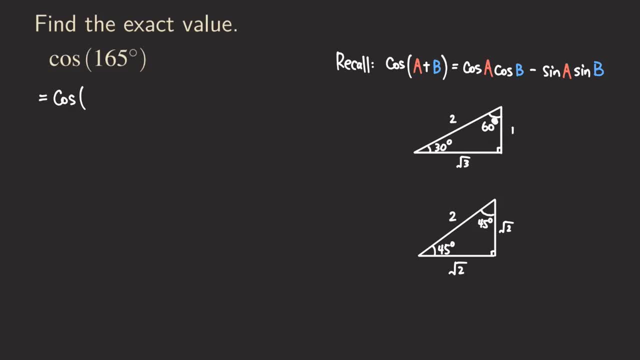 can think about multiples of those ones. Let's say, if we multiply the 60 by two, we're going to get 120.. So 120 would be a possible choice. So we can actually start with a 120 degree And then 165 minus 120 will give us the what the 45, right, so we are going to get 45.. 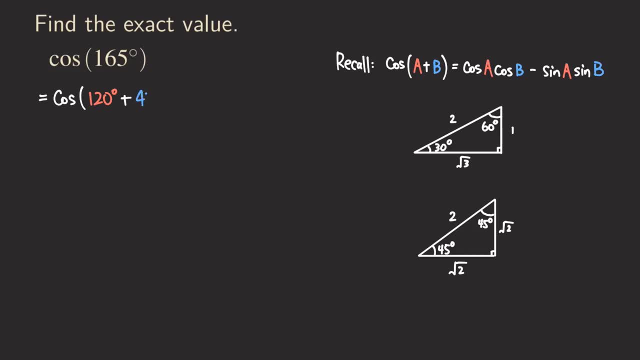 45 is one of the special ones, So we can actually use 45. So 120 plus 45 degree will give us the 165.. So now we have cosine of the sum of two angles so we can apply the formula, So we can actually start now. So let's just label this: this one is A and this one is. 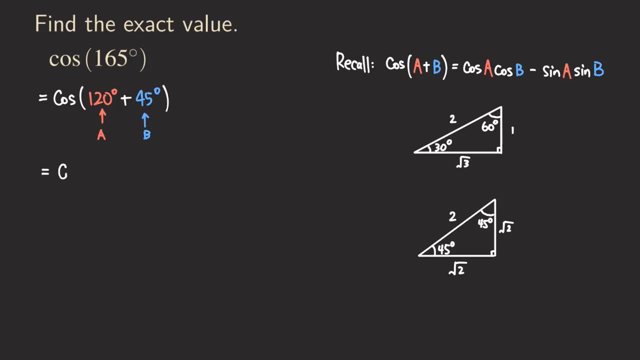 B: Okay, so we are going to write cosine of 120. So 120 over here. and then cosine of what? 45, right, the second angle. so we are going to get 45 over here. Then now, don't forget that this would be a minus sign here. 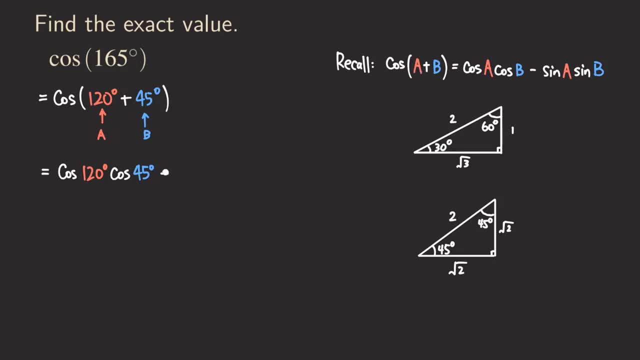 When we are applying the sum formula, this sign will be opposite of that one. So we are going to have the minus sign over here And then next we are going to get the sine of 120. So we have sine of 120 here, that's A and then sine B, right, so sine B would be sine of 45 degree. 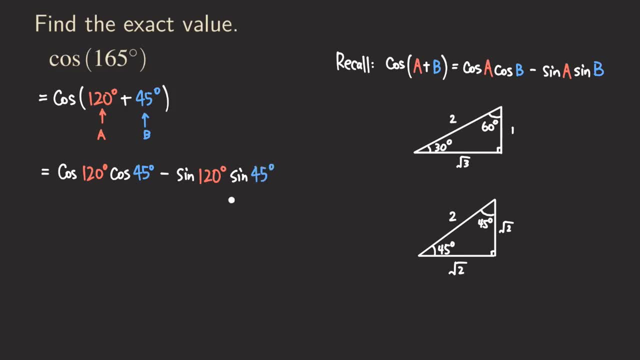 Okay, so now we have finished applying the formula. So now all we need to do is to come compute each part right here so that we can find the exact value. So what is cosine of 120?? Well, first we recognize that this angle, 120 degree, it's the angle with a terminal. 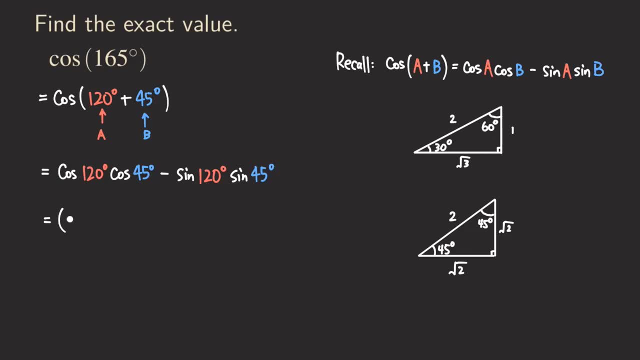 sign the second quadrant. So that means cosine will be a negative value. So we are going to put the negative first. And this 120 has a reference angle of 60, as you know, right? So in that case, what happens? what happens is that we can actually just refer to this. 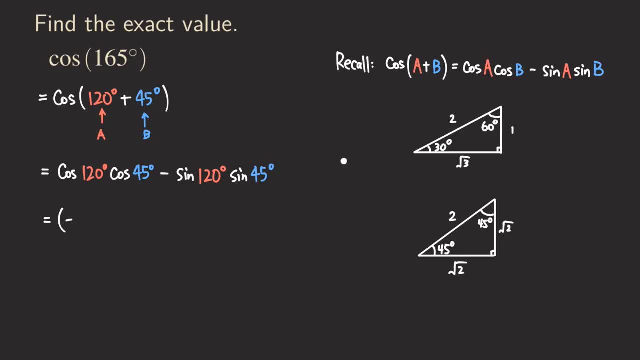 right triangle here and look at the angle 60. We are looking at cosine. cosine would be the adjacent over the hypotenuse. So we get 120.. So that means cosine of 120.. So we get one over two Now the difference between cosine 60, and then the cosine 120 degree. 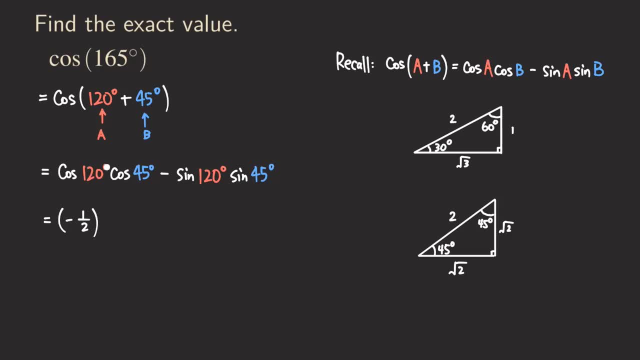 would be? what would be the sine difference, right? So because this has the terminal side in the second quadrant, so we have a minus sign right here. What about the cosine 45?? That's in the first quadrant, So that will be easy. So be positive. So cosine 45 would. 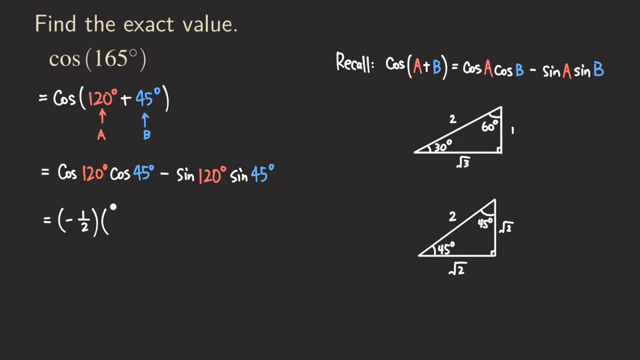 be looking at this angle here, adjacent over the hypotenuse. So radical, two over two. so we are going to have that Degree. And so again, this is in the second quadrant. So now what really happens is that we are going to um have a positive value, because that's a sign of one 20. So again, 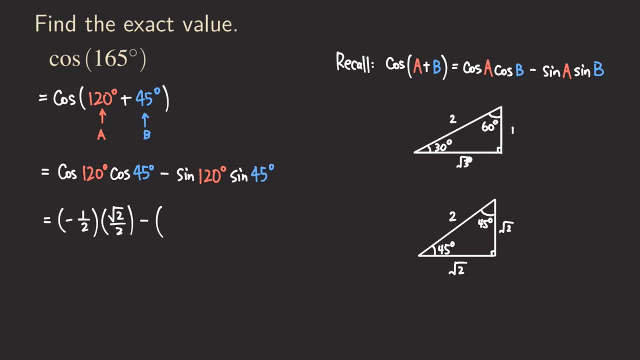 we are going to look at the um, the angle 60. So opposite over the hypotenuse, because that we're looking at the sign right, So opposite over hypotenuse would be radical, three over two and then times sine of 45 degrees, So sine of 45 degree, opposite over. 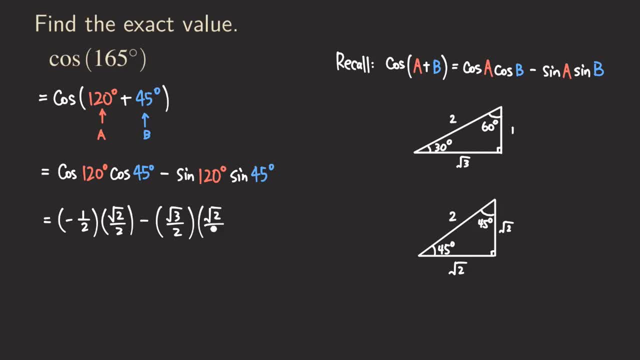 the Hypotenuse. So radical two over two, So radical two over two. So now we are actually ready. So we have what Negative radical two over four. And then there was a minus sign right here. Then we'll apply those two radical six over four, and that would be the answer of cosine of one, 65 degree. 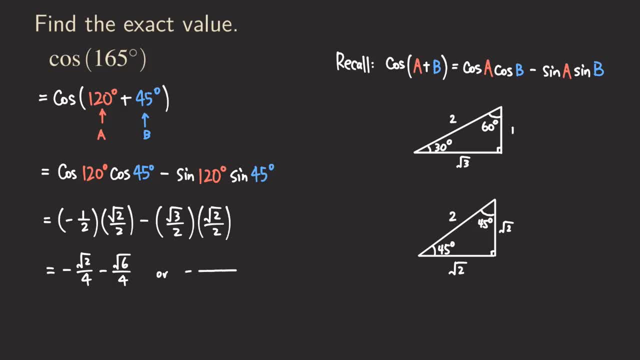 or we can actually put it as a single fraction. So we are going to factor all the negative sign in the front. So we are going to get radical two plus radical six and then over four. So now that would be our final answer. Okay, So we are going to look at another example. 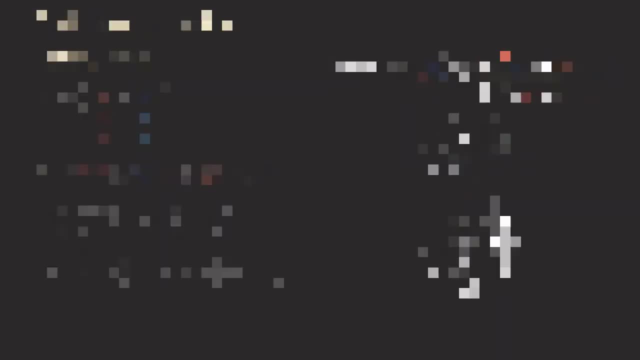 This time we are going to look at tangent. Okay, We already have seen how to use the sum formula for the sign of cosine. This time we are going to look at one with tangent And, as you can see here, this 345 degree, we can also write it as the sum of two special 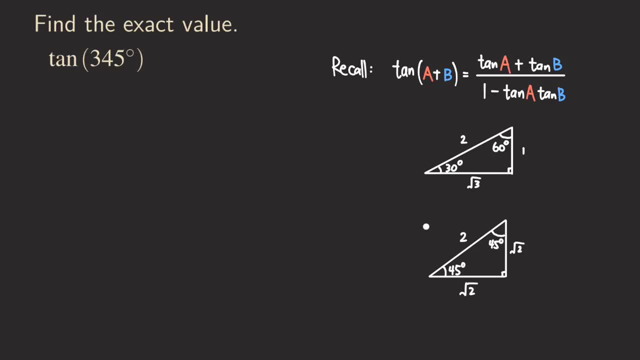 angles that we can actually just refer to those two special right triangles right here. So how do we do that? Well, the tangent formula looks a little bit different, So we're going to write it as a special angle And again, formula looks a little bit different It. 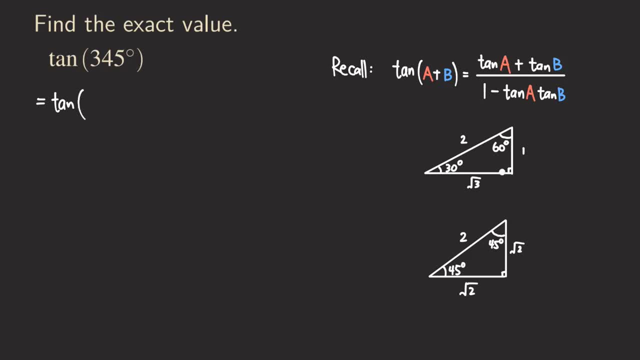 has a quotient over here, but that's not going to be really different. regarding on how we apply the formula, We still need to break this as the sum of two angles, right? So how do we break it? Well, one of them is that we recognize that there was a 45,, right So? 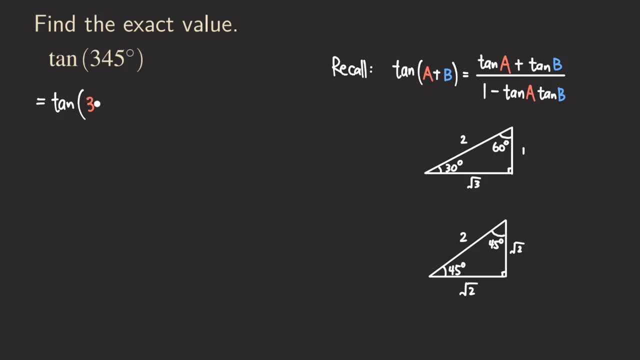 we can simply just write it as: what 300.. So 300 is a special angle, and then plus what- Just 45, right? So we are going to get 45,, which is the angle B, And so, as you can see, 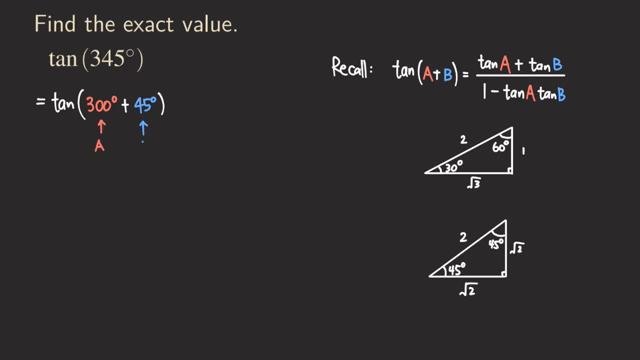 this one is a and then the other one is going to be B. Okay, so the next step is really just to apply the formula. So we are going to get: tangent of a is 300 degree. And then what about the B? the B is 45. So tangent of 45 degree. Then what happens is that we are going to get the 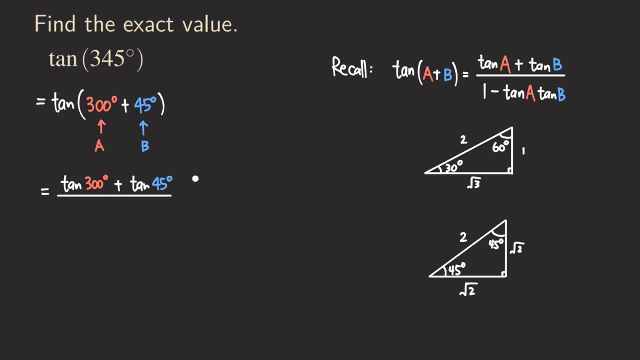 denominator now. So we are going to have what one minus the tangent of 300 degree And then the tangent of what is that? B? B is 45. So we're going to get 45 degree And then. so now we just compute each part. And then, how do we compute each part? Well, just. 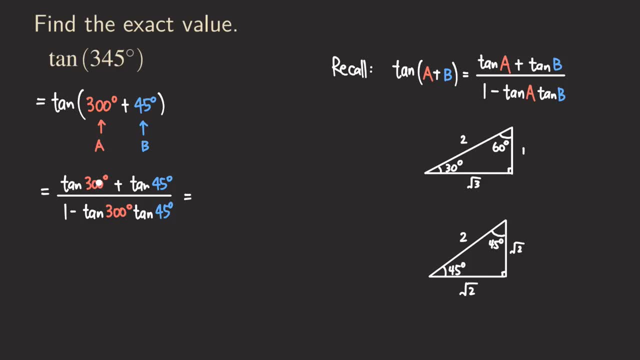 do each one separately. So now tangent of 300 degrees- 300 degree is actually has- is having a reference angle 60. So we are going to look at the 60 here. But we also need to pay attention to the quadrant. So it's terminal size in quadrant four. So what happened is that tangent will be a negative. So 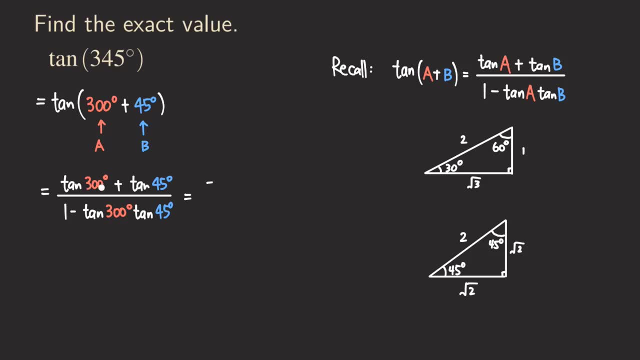 we are going to just put the minus sign there first and then tangent of 30. I mean tangent of 60 is what well? we look at the opposite over the adjacent. So opposite is radical three, adjacent is one. So we are going to get radical three over one, which is just radical three right. 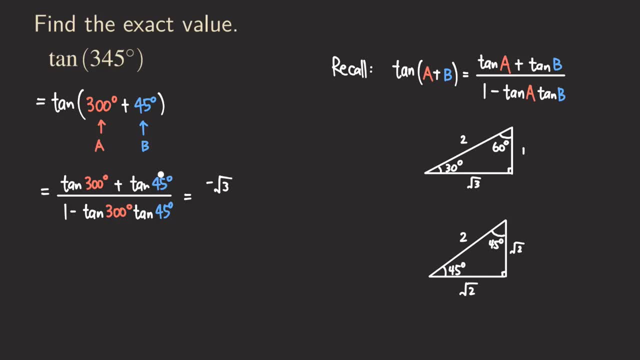 so radical, three over one, and then now plus tangent of 45. So this one is easy, quadrant one. So we get positive and then tangent is going to be what? 45? opposite over the adjacent, because we're looking at this angle right here, So opposite. 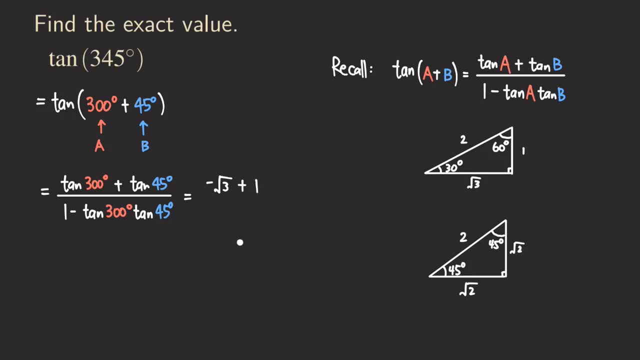 over adjacent radical two over radical two, which is just one. So we just get the one over there. Okay And so what about the denominator? So denominator is just the one over there, And then minus what tangent of 300 degree? we already figured out the answer over here, So we can just. 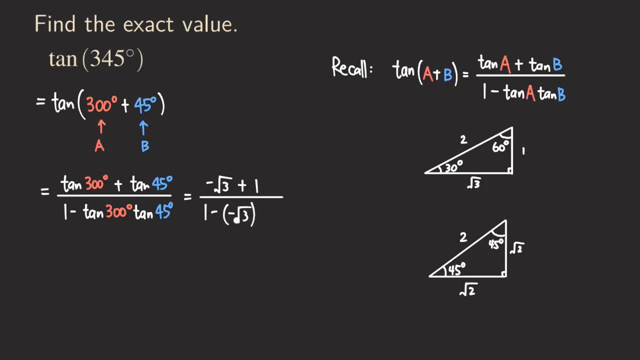 copy right. So we get negative, radical three. Now be careful with a sign, because this, this negative sign here, comes from the value, the tangent of 300 degree. but then there is another minus sign right here which comes directly from the formula. So make sure that you still write. 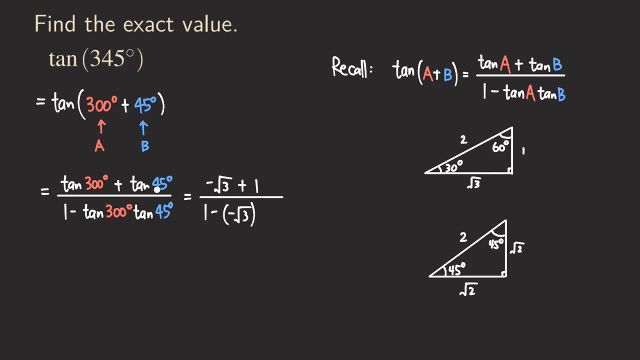 both signs right here. What about the tangent of 45 degree? the tangent of 45 is just one right, so we just just put the one over here. So now what are we getting? we are actually just getting one minus square root of three. I actually just reorder the terms. I put the one first and then minus. 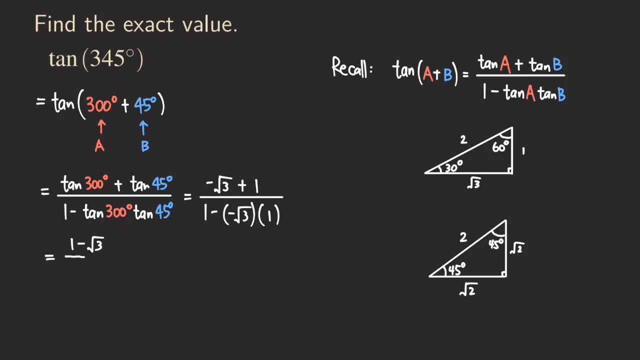 radical three, okay, And then in the denominator it would be one. and then this: this is negative radical three times one is just negative radical three minus minus. we have plus right, so we get one plus square root of three. Now that can be the final answer. But if you 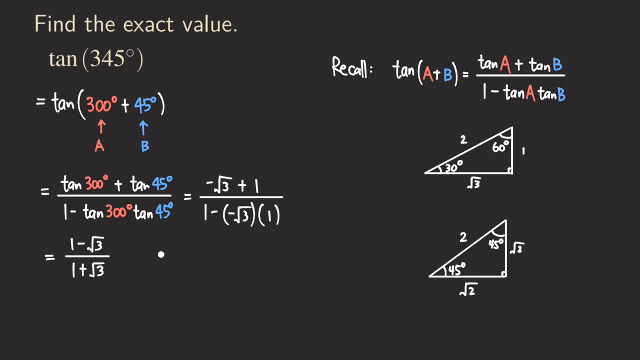 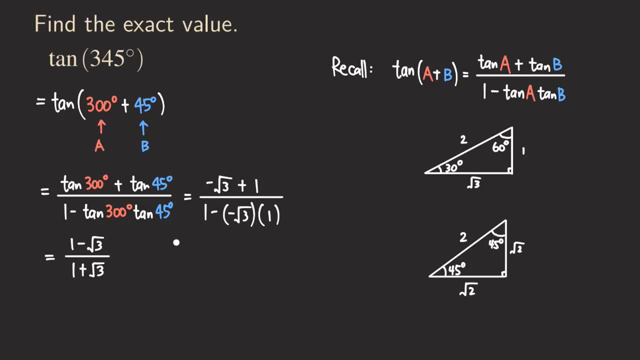 we are going to. well, let me just let me just write some calculation on the size. So we're going to get one minus radical three over one plus radical three. we can multiply the top and the bottom by one minus radical three. So we are multiplying by one. we are not changing the. 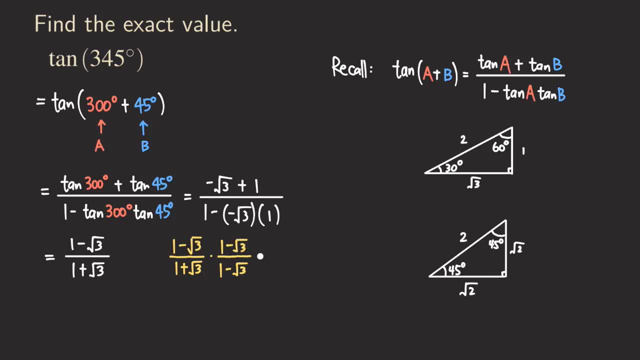 problem. Okay, So what happens is that the top becomes what one minus radical three, square. And then in the denominator we are going to just use the difference of two squares. formula: So: square, the first term, which is just just one right square, the radical three, we're going to get three and 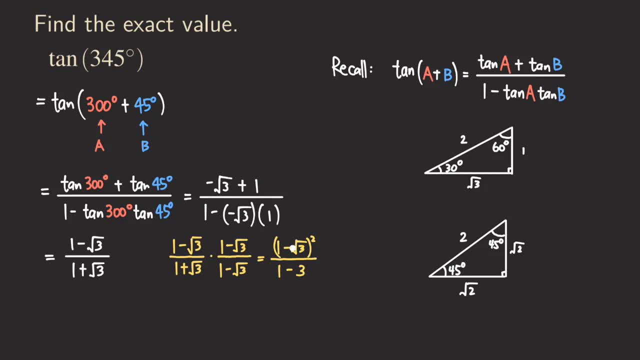 then we just put the minus sign right here. Okay, so now expand the top one. expand the top one is that we are going to get one and then minus two times those two, So we get radical three, and then plus square the radical three, So we're going to get the three here. So now the. 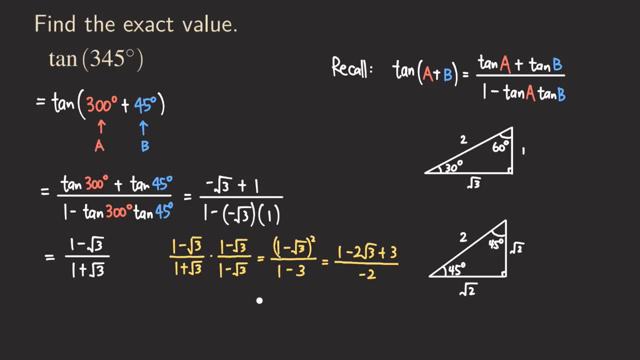 denominator. what about the denominator? just like the two. So continue with the calculation. we are going to get what one plus three is going to be four minus two, radical three divided by negative two. So you can actually break up the fraction to simplify this. 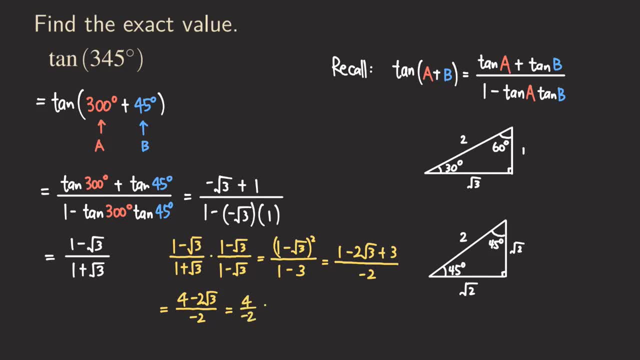 So we are going to get what? four over negative two, and then plus negative two, radical three over negative two. So cancellation. we're going to get what negative two and then cancel, cancel, those right. negative two, negative two. so we are going to get plus radical three. So those minus. 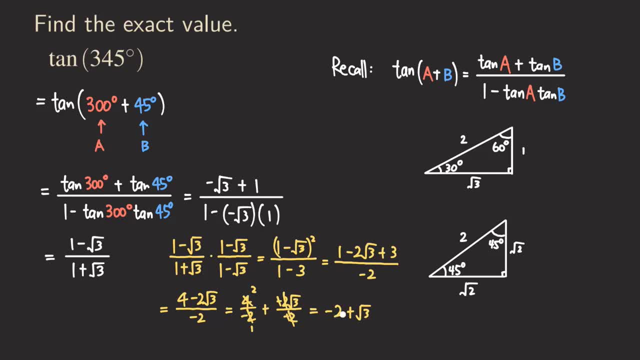 will also get canceled right. So we are going to get negative two plus radical three. So that is also another form of the final answer. So it's up to you which form they want to use, or depends on your requirement for your from your teacher. So we, either you can just write on this. 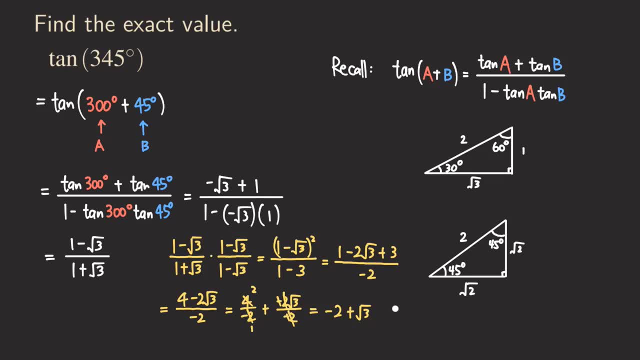 one or that one. Okay, so that's it for all those three examples. I hope that now you know how to apply the sum formula for the sine, the cosine or the tangent. Okay, so we'll do more examples next time. I will see you.